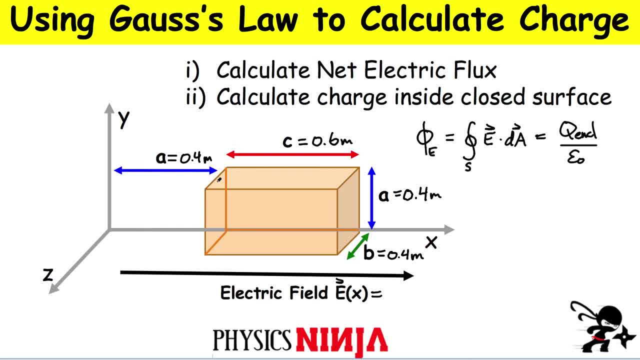 a closed surface, because that goes into the definition of Gauss's Law. So what we have here is a rectangular prism. I've given you the length of each side, So this surface over here is going to be a square. We have that. the height here is 0.4 meters and the width is 0.4.. The length now is 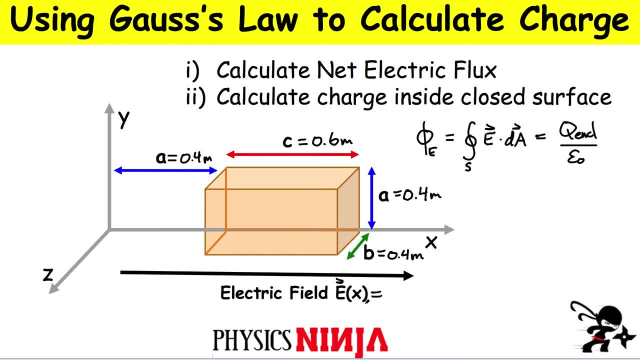 given by the letter C, and that's going to be 0.6 meters. Now, the other thing I'm going to have to give you is what is the electric field in space over here? So the electric field for this particular problem is only in the x direction. However, I'm going to give it a functional form. It could be a. 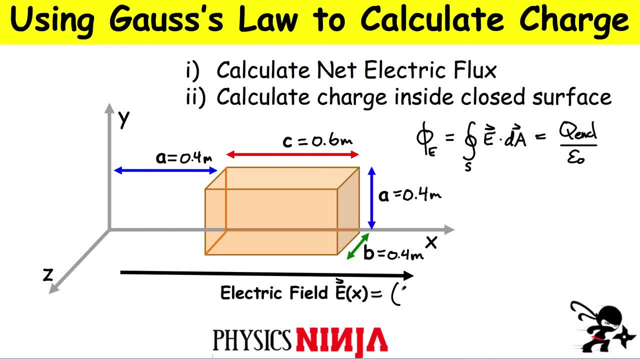 constant. We're going to make things a little bit harder for us here. We're going to assume that the electric field is given by this 3x plus 2x squared. All right, that's going to be the formula, And. 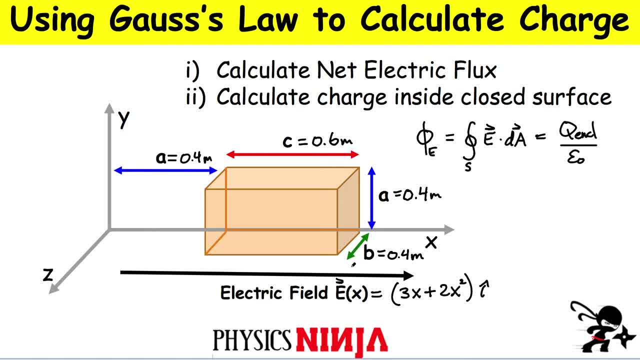 again, it's only going to be in one direction, So I'm going to give it the direction in the i-hat direction, which denotes the x direction. Okay, so this is kind of the problem statement. Now let's go back to our two problems and see how we 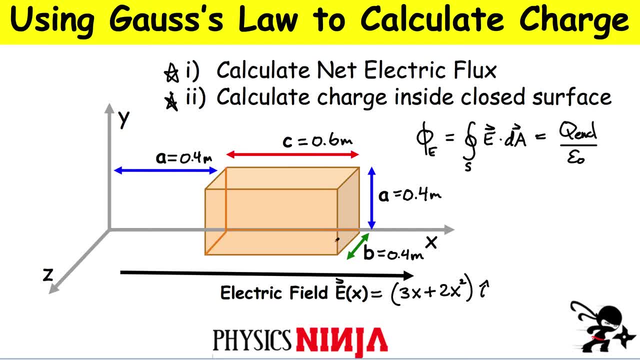 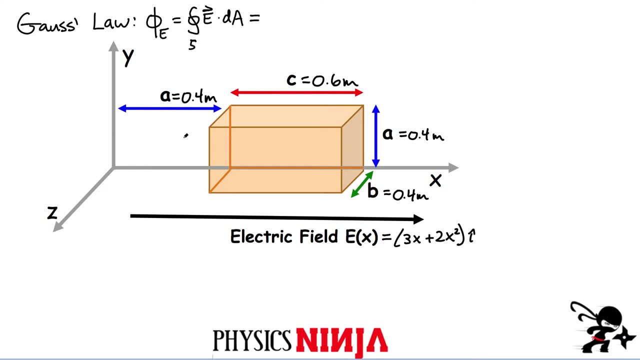 set it up to calculate what is the net electric flux through this prism and how do you calculate this charging closed. All right, so let's go to the next page and set this up. All right, so let's first start with the left-hand side of Gauss's law, which is this: integral over a closed. 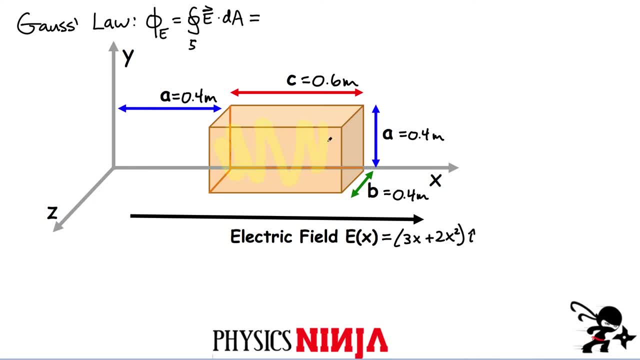 surface, And the closed surface is nothing more than the surface of my rectangular prism. Okay, so what we're going to do is you can basically split this up. Integrating over a closed surface means we're going to integrate over each surface of this rectangular prism. So let's start by. 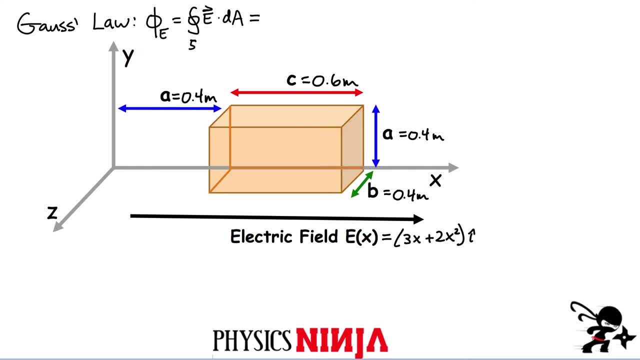 defining them. Let's try just using a marker over here. So the surface S1 is going to be the surface here. that's all the way. on the left-hand side We're going to call this S1.. Surface S2 is going to be on the other side, And then we can go ahead and label the four other surfaces- S3,, for example. 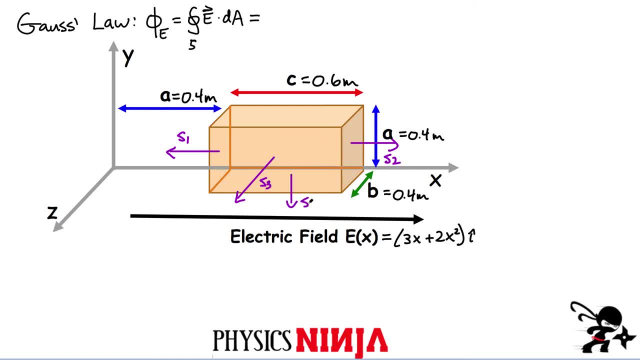 the front surface of this prism S4, the bottom S5, the bottom S6, the top S7, the bottom S8, the bottom S9, the bottom S10, the bottom S11,, the bottom S12, the bottom S13, the bottom S14,. the bottom S15, the bottom S16, the bottom S17,, the bottom S18,, the bottom S19, the bottom S19, the bottom S20, the bottom S21, the bottom S22, the bottom S22, the bottom S23, the bottom. 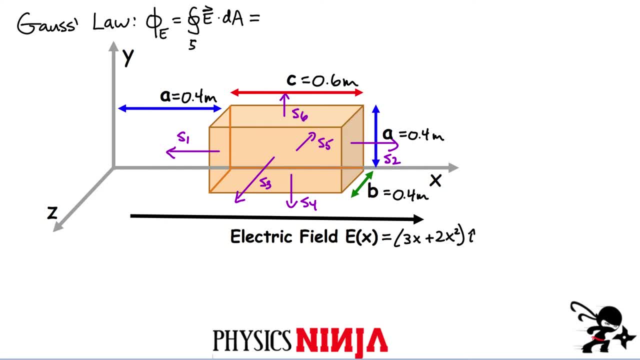 The top surface. let's call this S6.. Okay, so an integral over a closed surface, I can now simply write it as the sum of all the integral over individual surfaces. Okay, so that's going to simplify things a lot. It might not look like it, because now I have six terms to evaluate, but 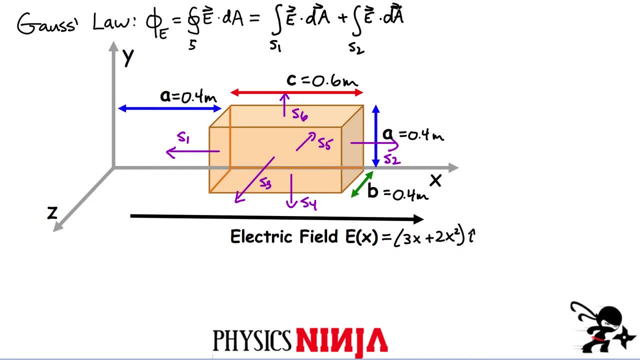 we're going to see that a lot of those terms are going to be equal to zero. So again, I have to integrate the electric field over the area of each one of those surfaces, And this is going to continue. I really have six terms over here. I'm not going to write them all, because they all look. 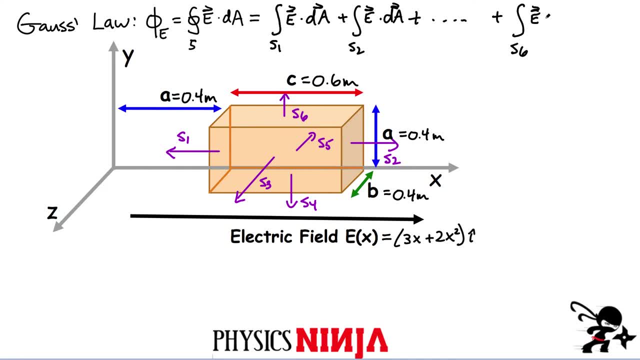 the same. So you just have to realize they're integrating over different surfaces. Now let's have a look at a few of those surfaces. Let's have a look, for example, at the surface S3.. All right, which is the front surface over here of this rectangular prism. All right, this is the. 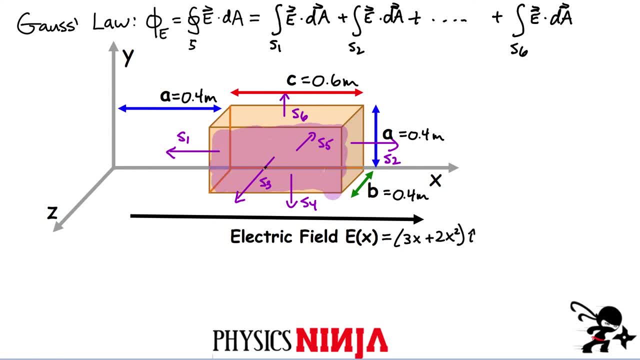 surface S3.. All right, this is the surface S3.. All right, this is the surface S3.. All right, surface that I'm interested in and it has an area vector that is pointing out of the page right because the area vector points perpendicular to the surface. okay, so for this particular case, 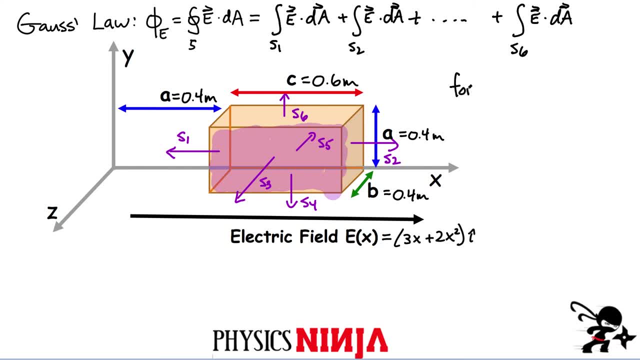 actually. let me write this down. so, for the surface s3, what we have is the area vector, or da, as a vector simply has a magnitude, da, but its direction, if you look its direction, is out of the page. that's what we're going to call the. 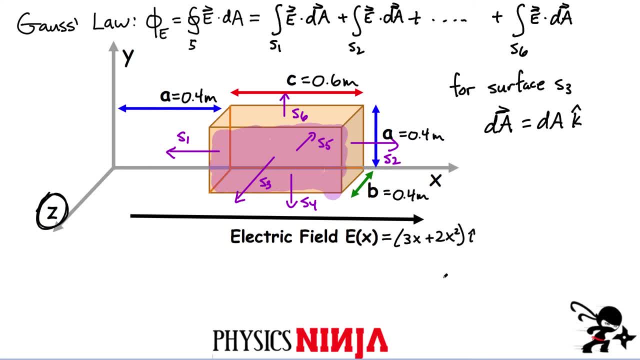 k-hat direction. okay, and now, if I was going to evaluate how much flux is actually going through this front surface, well, again, the whole term that you have to evaluate is s3. it's What is the electric field along that surface. Now, notice: the electric field here changes everywhere on the surface. 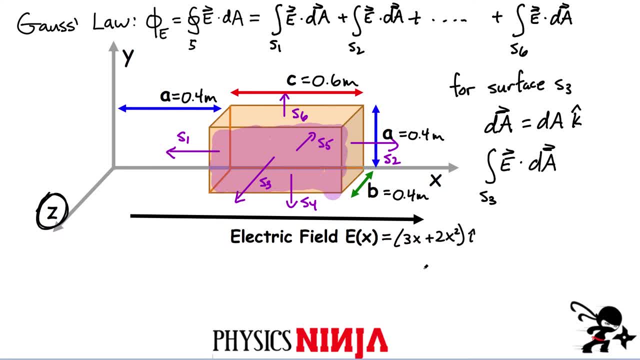 It's the scalar product with the area. Now, the scalar product: here you can simplify it right, Because you have to integrate over the entire area. The way you simplify a scalar product, it's the magnitude of one field, It's the magnitude of the other vector, multiplied by cos of the angle between both of those vectors. 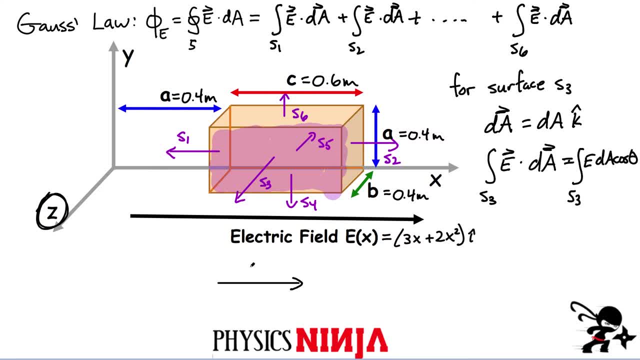 However, look at what we have. We have an electric field which is always along the x direction- That's given by this term right here- And what we have is an area vector dA, which is going to be in this direction over here, right. 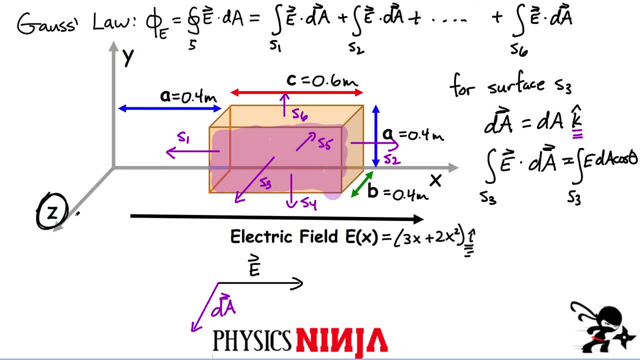 That's what we found. dA is along the z direction, So that means that the angle between both of those vectors is always 90 degrees. If that's the case, that means that this integral right here has to be equal to zero. 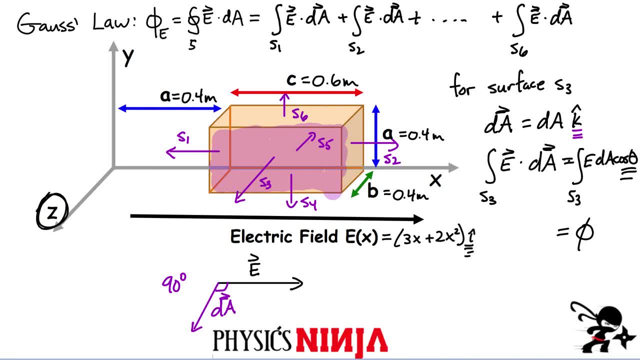 Because the angle here is 90 degrees and cos of 90 gives me zero. So that simplifies our life quite a bit. You're going to notice that you're going to get the same thing for S4, for S5, and S6. 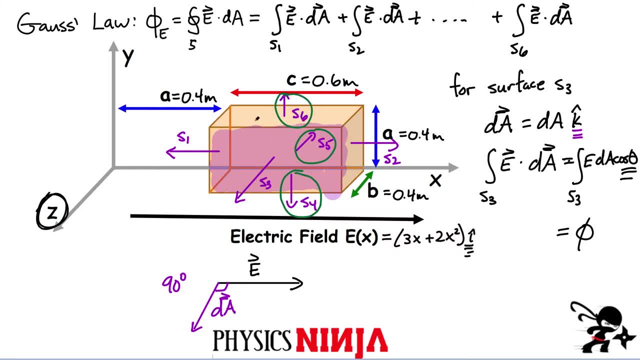 All of these terms. there is no electric flux going through any of these surfaces because of this scalar product right here, Because for each one of these we're going to have theta equals to 90 degrees And therefore you don't have to consider it. 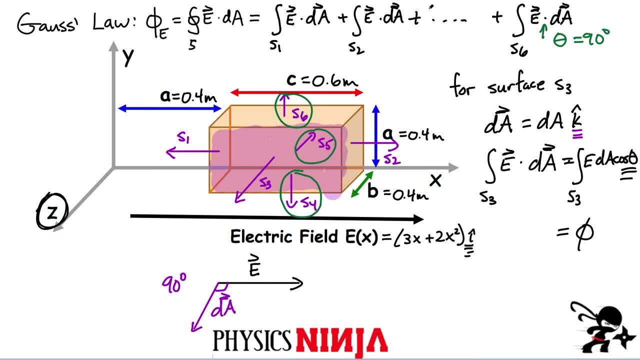 So that That really simplifies what our total electric flux is. because we don't have any of these terms anymore, We're only left with two terms: This one and this one. All right, so let's first start with this first term here. 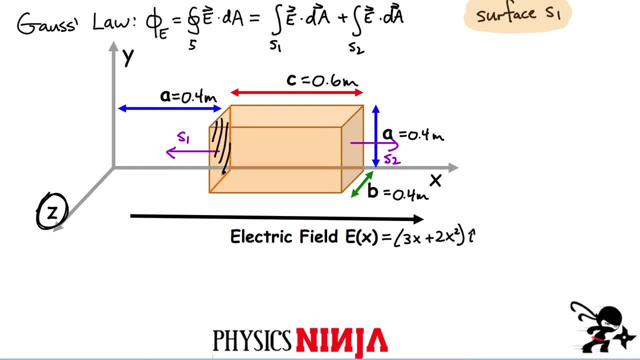 So we're going to be integrating over this area over here. Okay, so we have to define all the terms. First thing you want to know is: what is the electric field everywhere on the surface over here? So at the surface S1, what you have is that, the value of x. 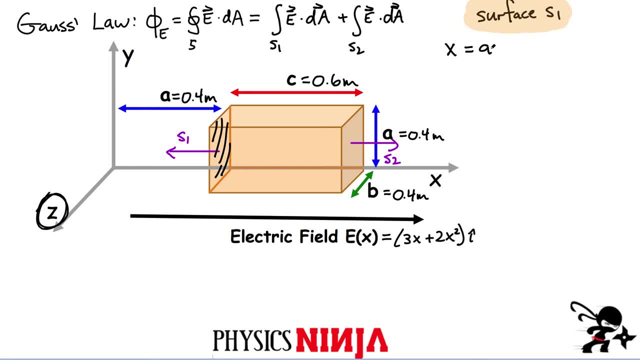 everywhere, for the surface is simply equal to a and it's equal to 0.4.. So what does that mean for the electric field? Well, the electric field expression is right there. So that means that everywhere on the surface, the electric field, since it only depends on x. 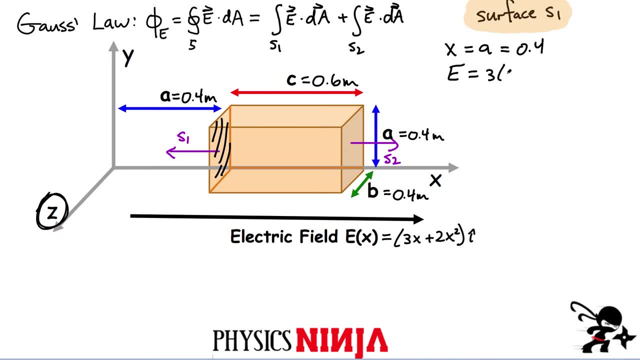 it has the same value. So you can just substitute in the value here 0.4 plus 2, and this is 0.4 squared. Now again, this is a vector quantity and that's going to be the direction of the vector. 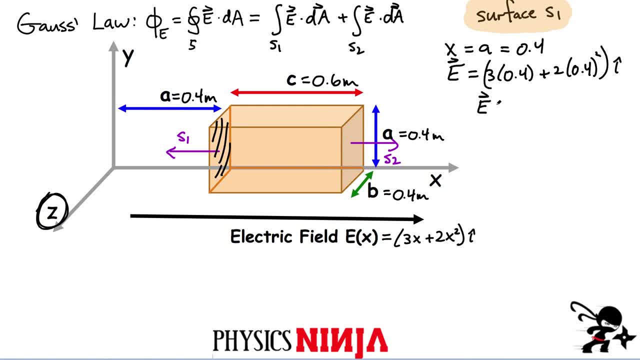 So what you can do now is just substitute that inside your calculator and you're going to find a magnitude of 1.52.. That's in newtons per coulomb, and the direction is going to be in the i-hat direction. 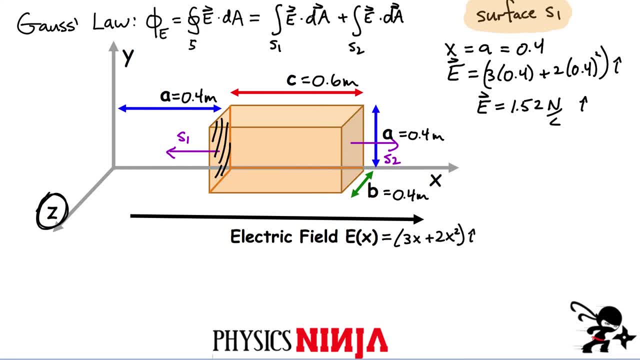 All right, so that's what we need, And the other term that we need is this: area vector. Well, what is the area vector? The area vector is basically a vector that points in a direction that is perpendicular, right? So I can write it as something like this: 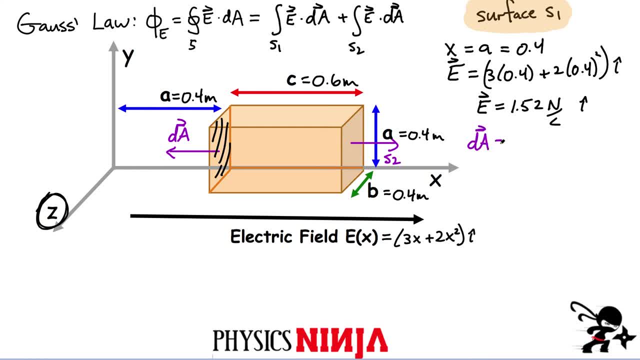 Now, if you write it down as a vector, it looks like this: It has a magnitude, The magnitude is simply dA, and the direction of that vector is well, it's opposite of the electric field, right? I would say it's in the minus i-hat direction. 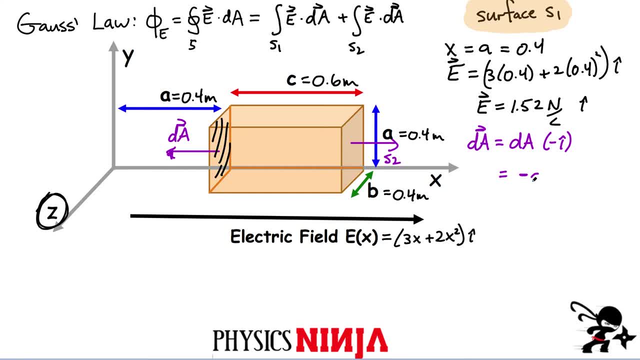 So if you want to write that kind of neatly, maybe just put the negative in the front: dA and i-hat, All right, that's how you write the vector. Okay, so we have our two terms here, and now we want to evaluate those. 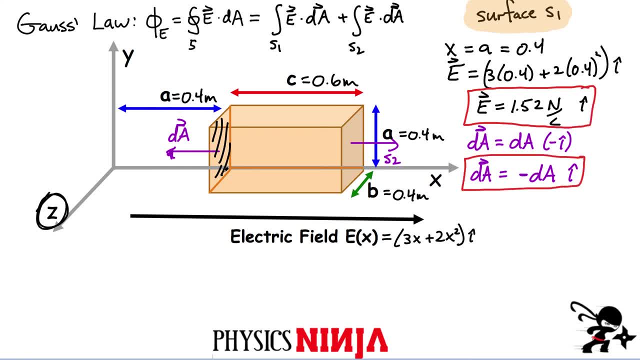 Inside the integral. Now it turns out to be pretty simple, because the electric field is uniform everywhere along the surface. So that means that anything that's a constant, you can basically take it out. So let's go ahead and evaluate this first integral term. 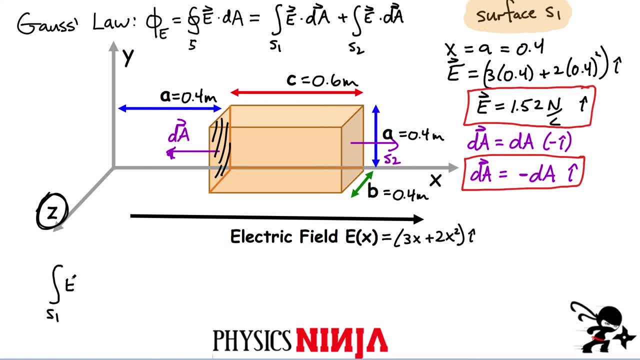 So I'll write it down first: S1, E, dot, dA, something like this. Now we substitute in all the vectors, So I want to integrate over the entire area S1.. And I have my, And I have my magnitude, which is 1.52, multiplied by i-hat. 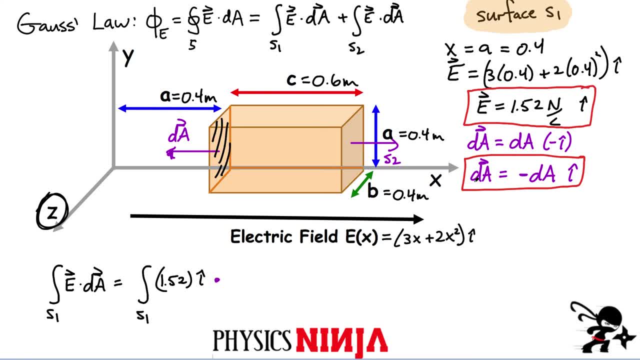 And that will become a scalar product with the other vector. The other vector is going to be- well, let me open up a square bracket here- negative dA And that is multiplied by i-hat. Okay, so let's factor out the constant term. 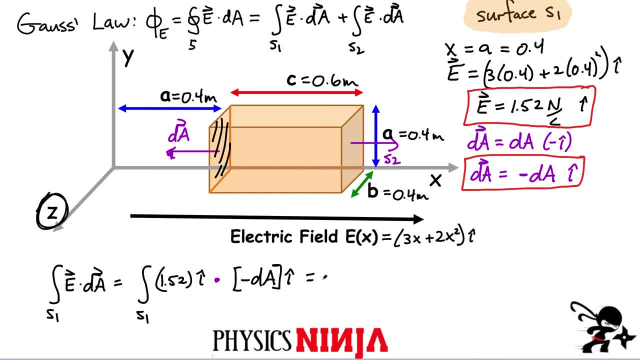 The constant term is that magnitude of the electric field over here. This is 1.52.. And I want to integrate. now There's a negative in the front that comes out, That just comes from this term over here And the left. what I'm left with here is dA S1.. 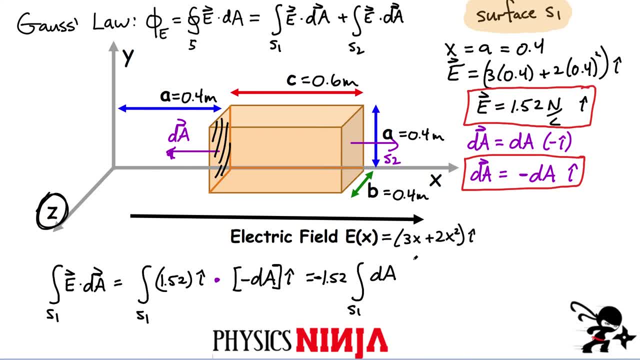 And I have an i-hat dot, i-hat. Okay, well, i-hat dot, i-hat. you should remember that- one That is simply equal to 1, so you don't have anything to worry about for that one. 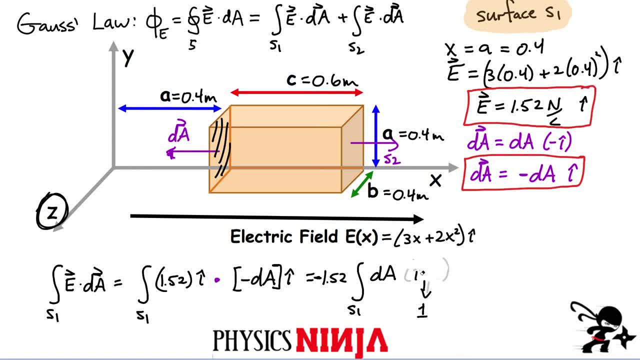 That's very, very easy. Let's just kind of eliminate that term. That's just the 1. Just erase it And all I'm left with now is simply integrating over the entire area. All right, the constant electric field magnitude left. 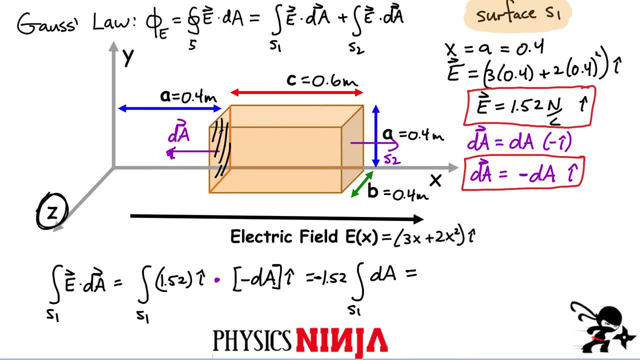 So what we're left with now is just the integral over the area. is just the area right Or the integral over that surface simply gives me the area. So at the end we're left with minus 1.52 and multiplied by the area of this surface. 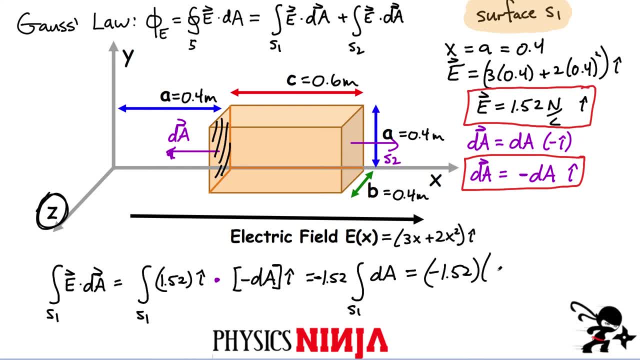 The area of that surface is going to be the height multiplied by the width, That's A multiplied by B. Okay, and both of those are the same value, since it's a square surface. So at the end you get minus 1.52, 0.4 squared. 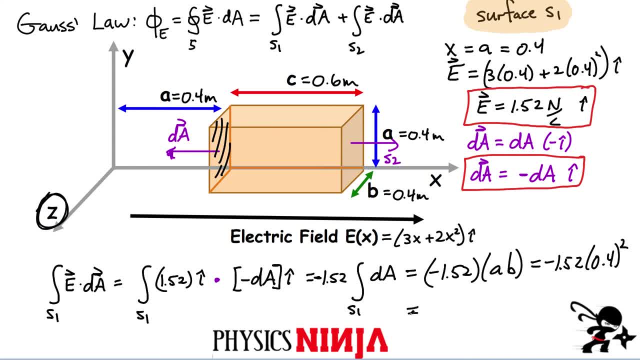 And we're left with that, this first term right here. at the end of the day, this will give me negative 0.2432.. Okay, and that'll be in units of well, whatever the electric flux units are. For now I'll just write it as: 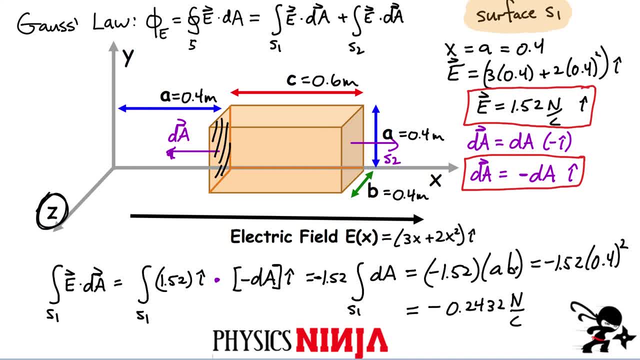 The electric field units, which are newtons per coulomb and multiplied by meters squared. Okay, so that is this first term that we've just evaluated. Now the second term, we're going to do in a similar fashion, And the only difference is that the electric field has to be evaluated at a different position. 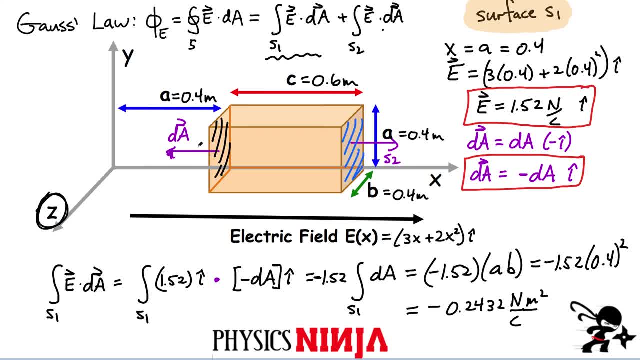 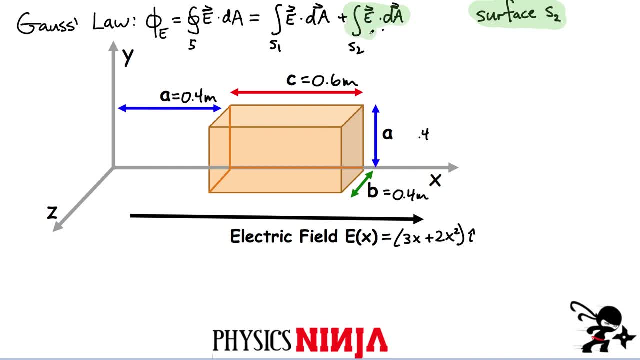 All right. the electric field now has to be evaluated at this position instead of the first surface, So let's set that one up, All right. so now we're interested in The second term. over here it has a similar form, And the surface that I really want to integrate over is this one, right? 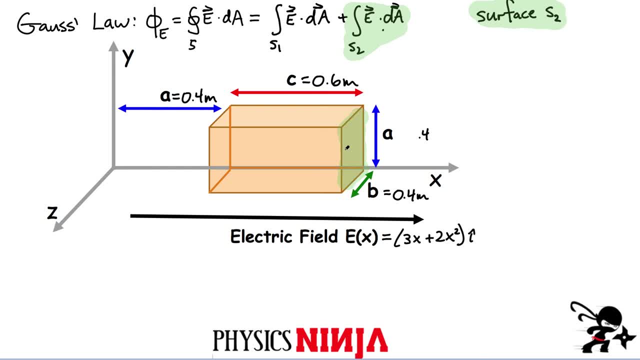 The other side of my prism, So that surface is at a different position and it has a different area vector right, And I have to integrate over this entire area right here. What else? Well, we also have that the surface is located at a distance of 1 meter from the origin over here. 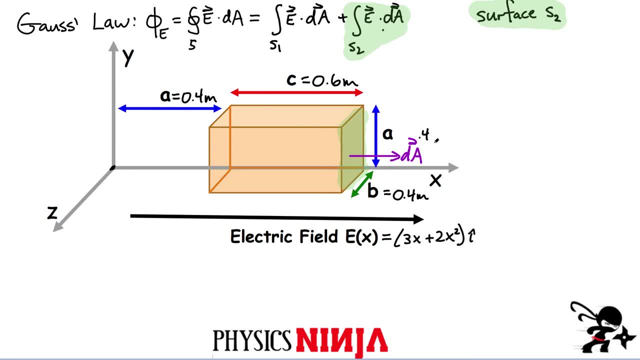 Right, that's the distance over here, That's the value x. So when you Actually calculate what is the magnitude here at this position, where x equals to 1 meter, That's the position of the surface which you're going to end up getting- is well. 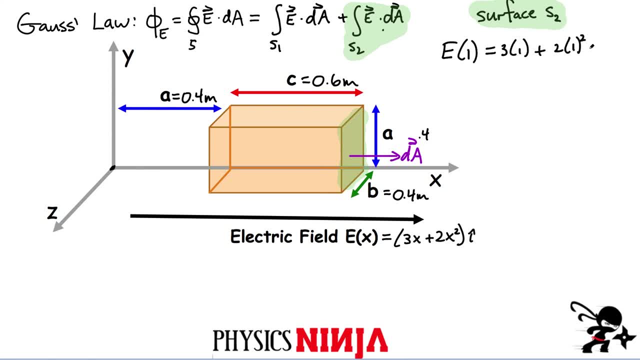 3 times 1 plus 2 times 1 squared, And everything still is in the i-hat direction. So that simply gives me 5, right, 5 newtons per coulomb, And again it's in that direction. 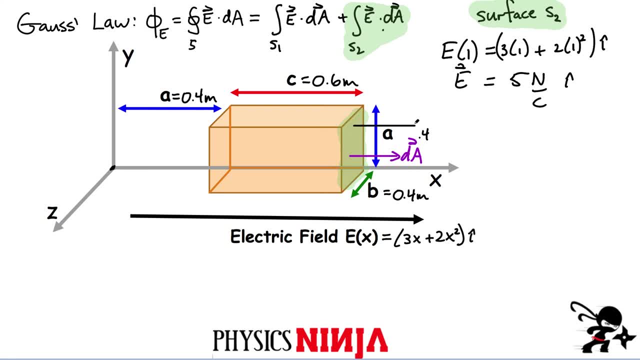 That's our electric field. So actually, if you plot the electric field right here, you should have it in this direction here. All right, so what are we left with? We have to find what is this area vector over here? So the area vector should be equal to the magnitude and multiplied by the direction. 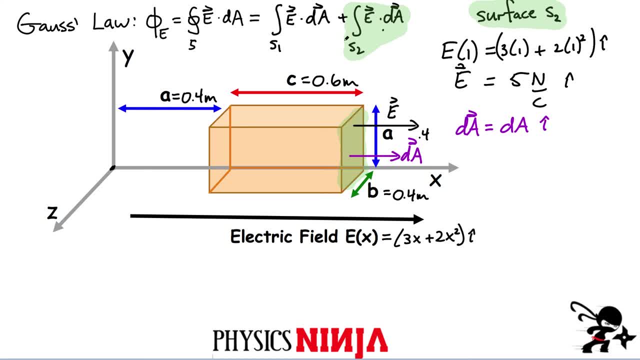 Notice it is now parallel to the electric field, So that's going to simplify this term. So at the end, this is what our integral looks like. So we have the integral over S2 of the electric field scalar product with the area vector. 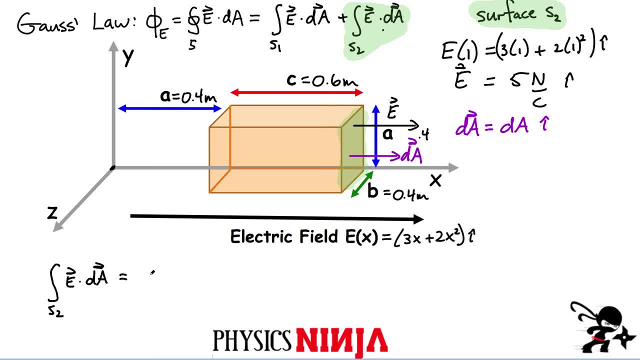 Okay, what we're left with here is simply going to be 5.. S2, we have our vector 5. That's the electric field and scalar product. with dA and i-hat, We have another pair of brackets over here. 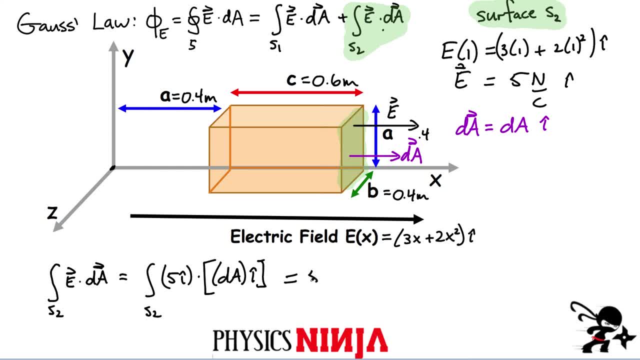 You see the 5 I can take out of that integral because it's constant And I have an ii term. This simply also reduces to 1, just like I had before, And what you're left with is simply the integral over the surface. 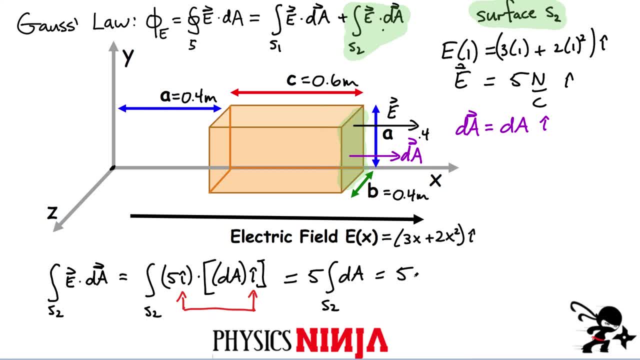 And that's it, And that is simply 5 multiplied by the surface. That surface is again A times B, right? So we have 5 multiplied by 0.4.. And since it's a square surface, it's 0.4 again. 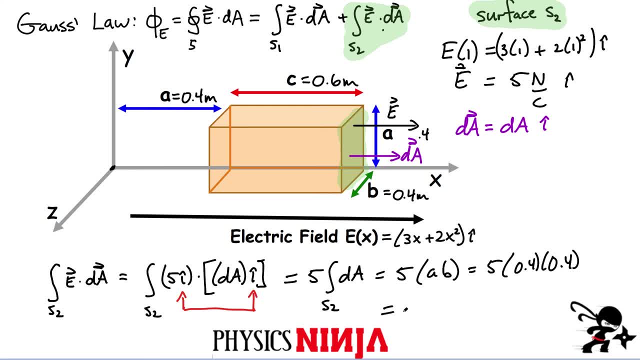 So that means that this second term here gives me a value of 0.8.. Again in the same units, Newtons per coulomb multiplied by meters squared. We now go back to our first question: Calculate the net electric flux. 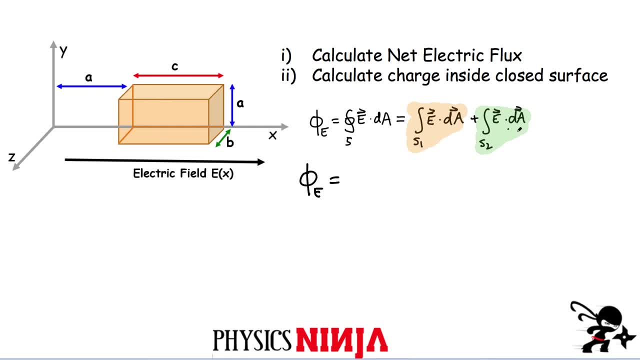 Well, we did quite a lot of work here. So the net electric flux again reduced to this. adding both of those two terms together, That's all we have. So the first one was negative right The integral over the field in that area, 0.2432.. 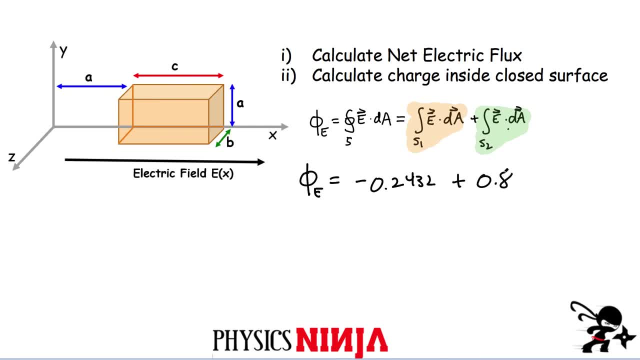 And plus the second term, we had 0.8.. So at the end our net electric flux should give me 0.557.. Again, newtons per coulomb. Newtons per coulomb meters squared. Okay, that is question one. 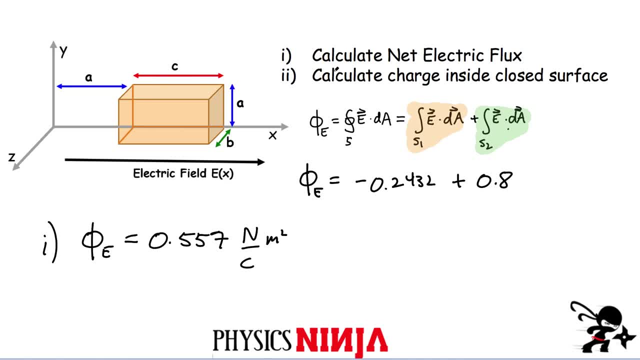 That was quite a lot of work. Question two is a lot easier. right, Calculate the charge inside the closed surface. Well, for that, all you have to do now is simply apply Gauss's law to this problem. All right, Gauss's law, remember, stated that if you know the net electric flux through a closed surface, 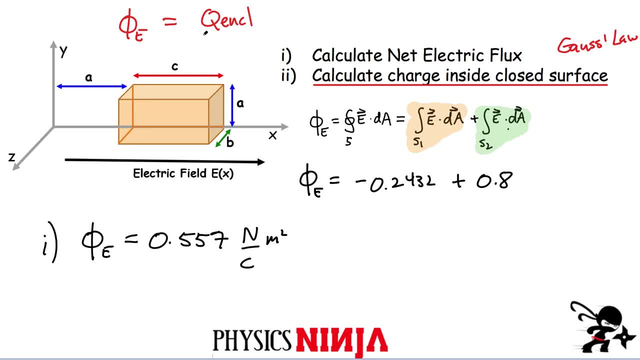 that is simply equal to the amount of charge that's enclosed divided by the net electric flux. This is divided by a constant. This is a permittivity of free space. You just look that up in your textbook So to find the total charge enclosed. all you do is just bring this on the other side. 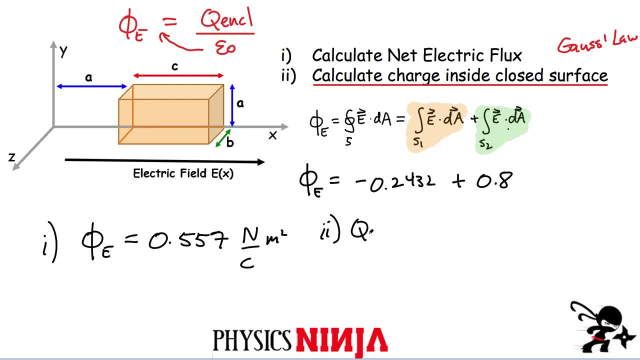 and you can right away just write down that the total charge enclosed is going to be equal to the total flux going through that closed surface multiplied by epsilon zero. So that's it. We're off to the races now. So you write our total flux, which is 0.. 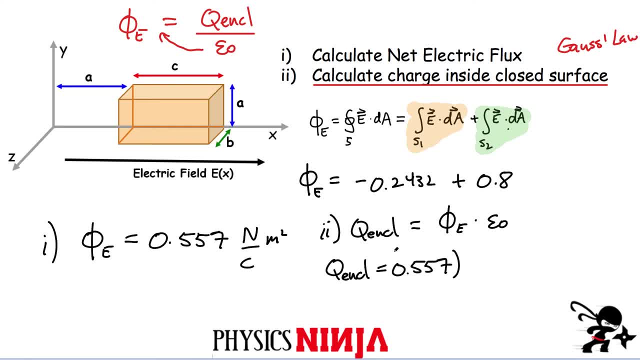 Roughly 5.57, if I round that and multiplied by the permittivity of free space- You look that one up in the textbook- 8.85 times 10 to the negative 13.. Again, all of this is in SI units, so we're good. 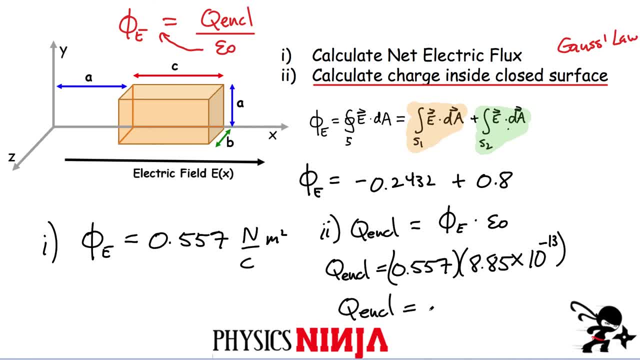 You carry out that multiplication in the calculator and you should get something that is approximately 4.93 times 10 to the negative 12.. And that is measured in coulombs. So that is how much charge is enclosed in that surface. 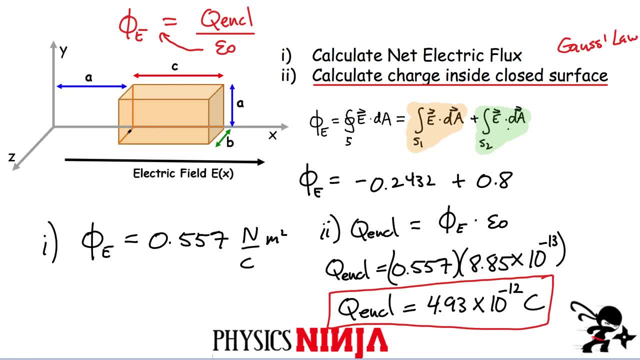 And we used Gauss's law in order to find this. Okay, Anyway, that's it for this problem, folks, Hopefully you can carry out the steps now. Okay, notice some of the simplifications In many of those surfaces, the flux going through that surface is zero. 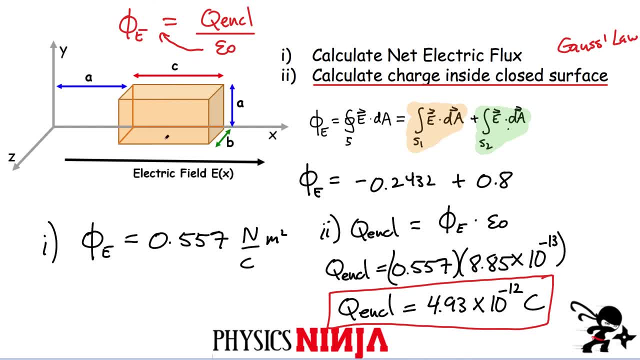 because the area vector and the electric field are perpendicular to each other And we were able to simplify the problem as to integrate the flux. So we're going to do that, We're going to do that, We're going to do that. We're going to be integrating over only two surfaces of this rectangular prism. All right, thanks for watching folks.